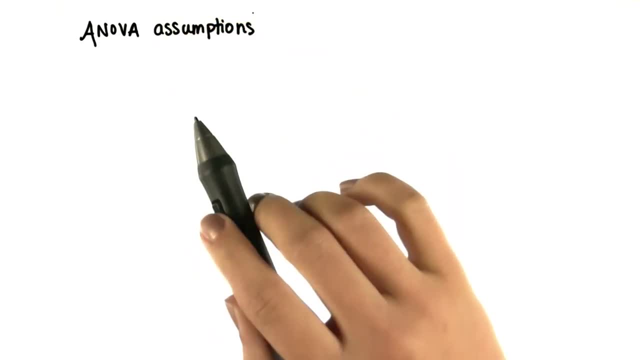 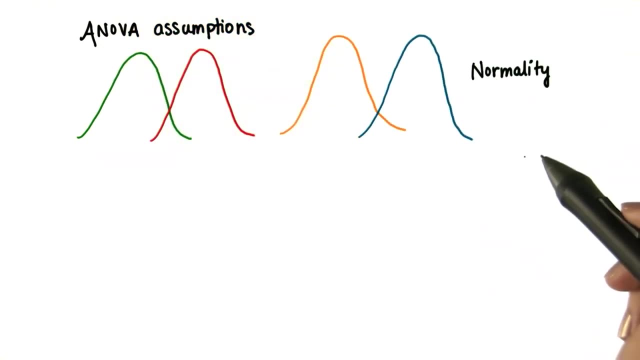 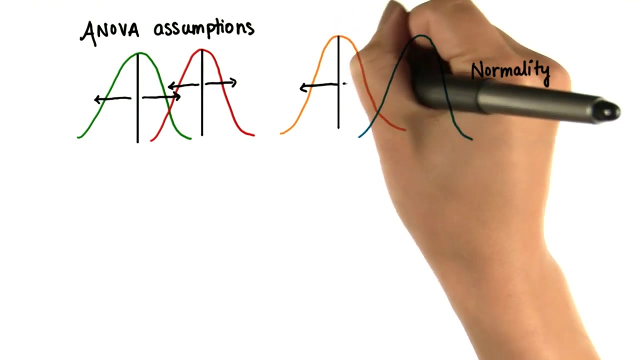 Finally, we need to make some assumptions in order to use one-way ANOVA. The first is normality: All the populations from which the samples are from are normally distributed. Another is homogeneity of variance: The data come from populations that have equal amounts of variability. And finally, independence. 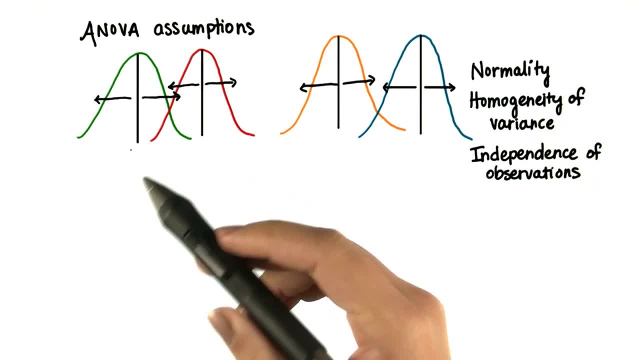 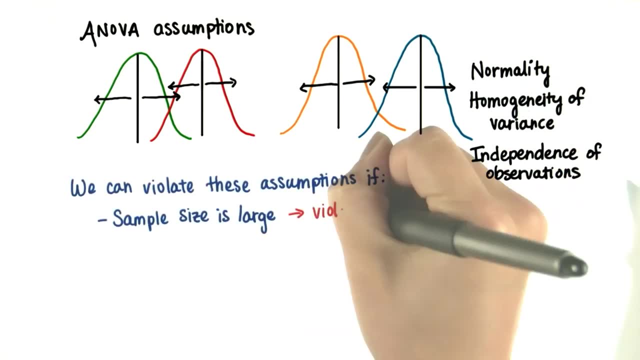 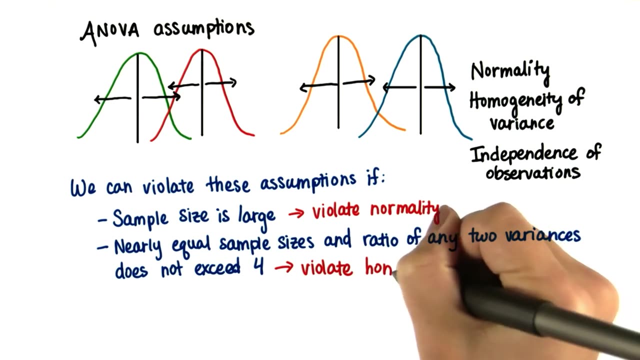 of observations. The results found from one sample won't affect the others. However, we can violate these assumptions under certain conditions. We can violate the normality assumption if the sample size is large. We can violate the homogeneity of variance assumption if all the samples have nearly equal sample. 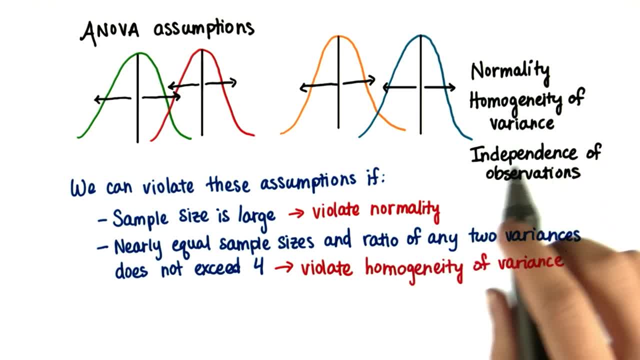 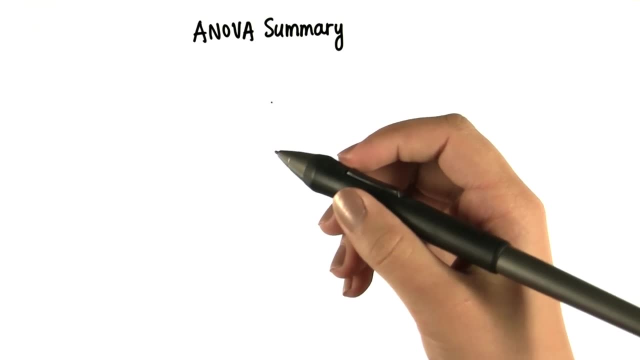 sizes and the ratio of any two variances does not exceed four. We have to maintain independence of observations, but we can use random assignment to conditions to help us meet this assumption. Let's do a quick summary of ANOVA to wrap up this lesson. I'm not actually going to wrap this. 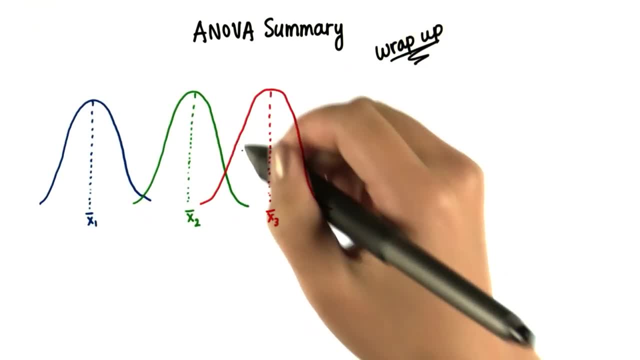 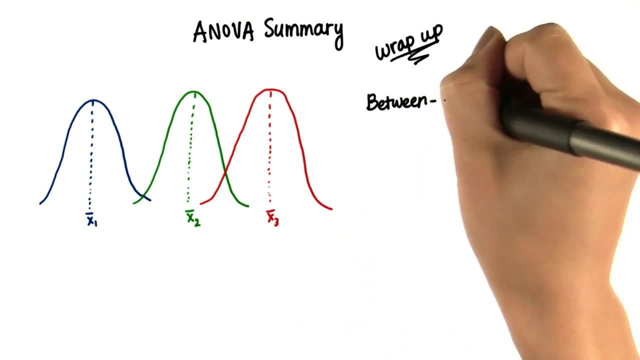 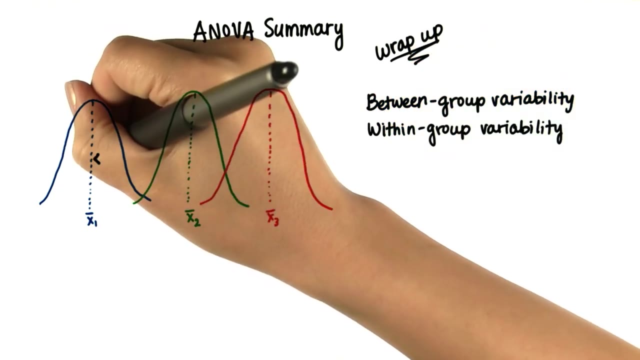 time, though We're just going to wrap up the lesson. If we have three or more samples and we want to know if any two of them are significantly different, we look at both the between group variability and the within group variability. Between group variability is a measure of how, spaced apart, these sample means. 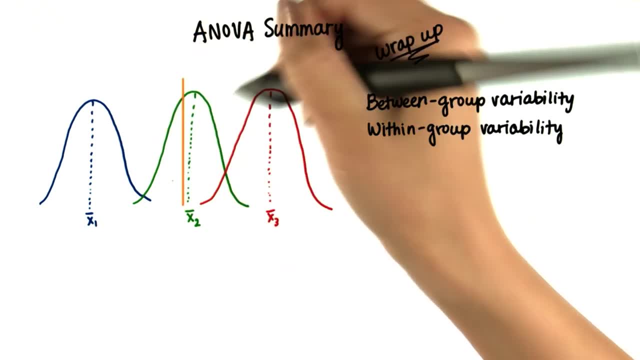 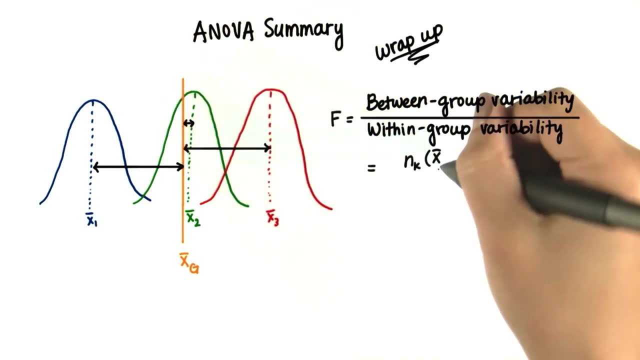 are from each other. And we do that by finding the grand mean, which is the median, and each square deviation from the grand mean for each sample mean. We multiply each sample size by the square deviation of each sample mean from the grand mean, Then we add them up, Then we have to look at the within group. 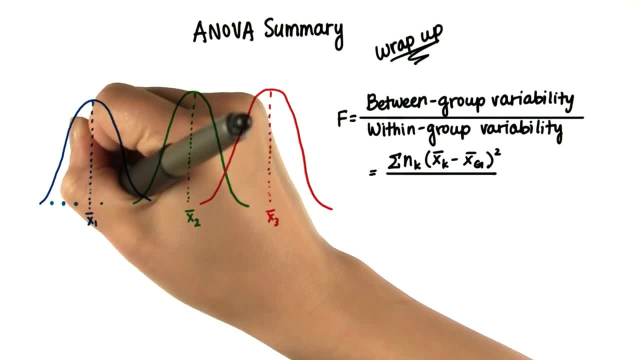 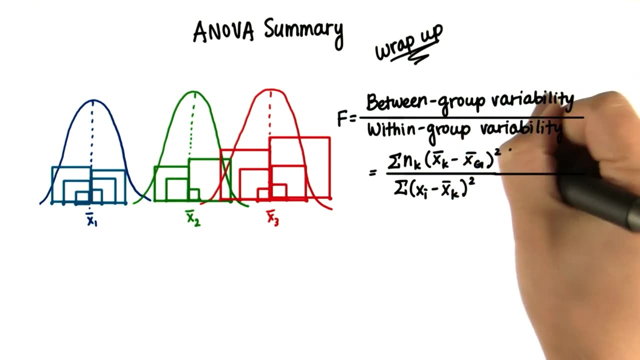 variability, which is essentially the square deviation of each value in each sample from the respective sample mean. So we add up the square deviation of each sample mean And then we have to find the average sum of squares for each by dividing by the degrees of freedom. In the case of the between groups, this is: 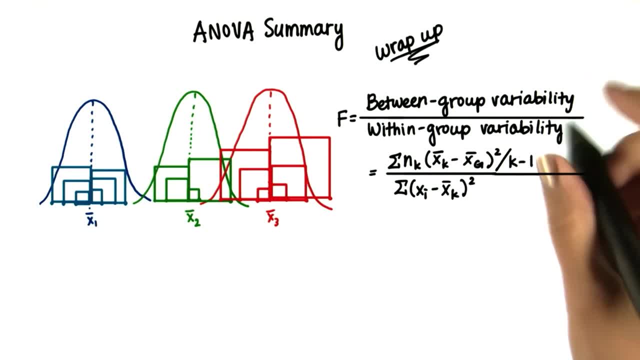 the number of samples minus 1.. And for within groups, this is the total number of values minus the number of groups. This is the same as adding the degrees of freedom for each group. There we have our F statistic And if we look at the 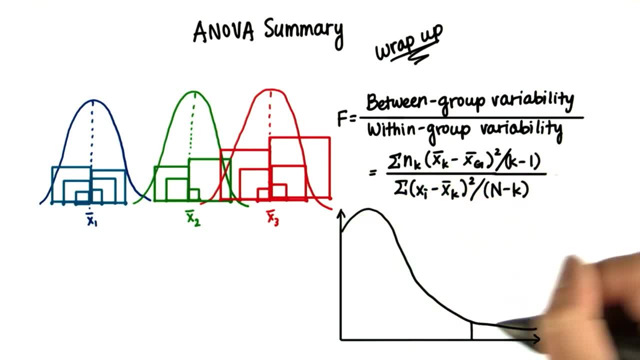 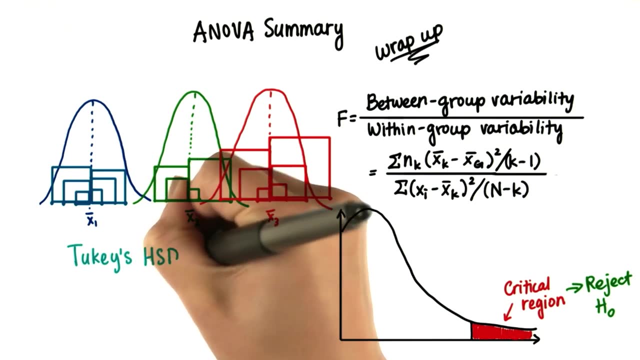 critical region past the F critical value, we'll reject the null. After making a statistical decision, we can use the multiple comparison test, one of which is Tukey's honestly significant difference, Which is a value that, if any two sample means have a difference greater than that value, they're considered. 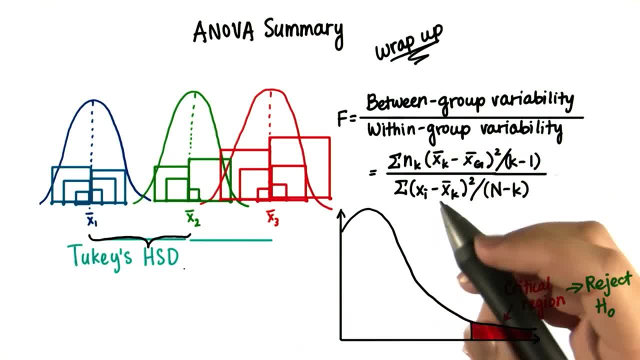 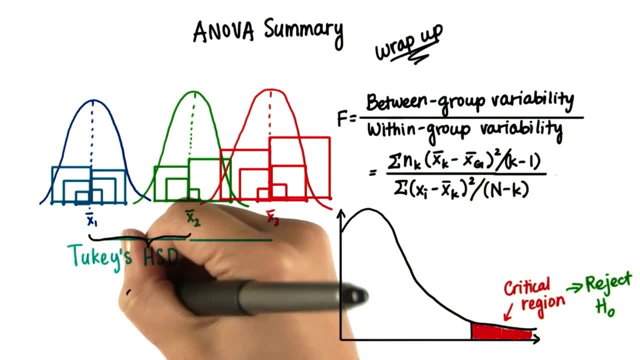 honestly, significantly different. You've also learned how to determine what proportion of the difference between means is due to the independent variable. That's eta squared And that's a wrap. 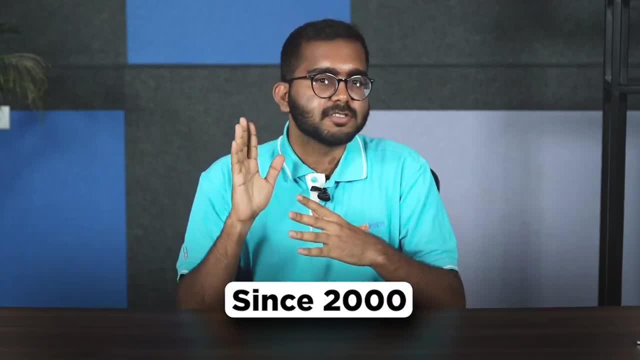 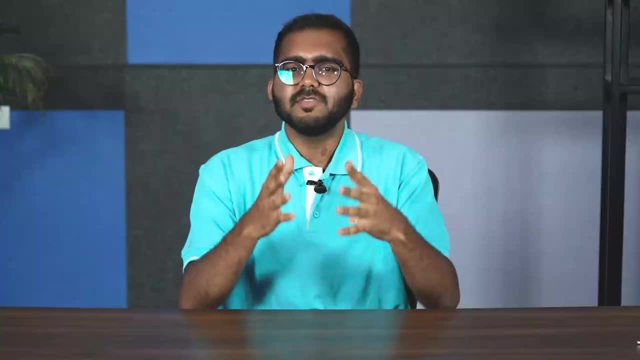 The growth of AI startups accelerated 14 times since 2000.. Pretty good news. right From healthcare to robotics, agriculture to education, AI is impacting every industry. This will simultaneously increase opportunities in AI. Through the use of technology, businesses are able to improve. 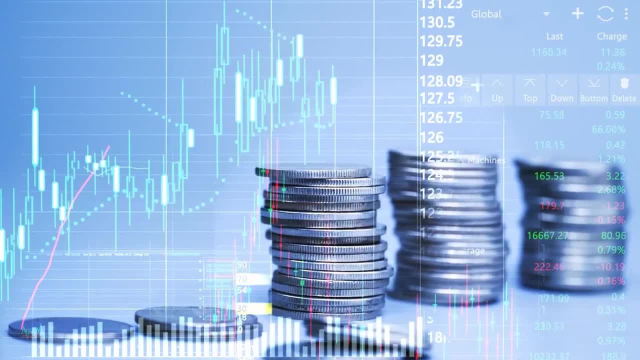 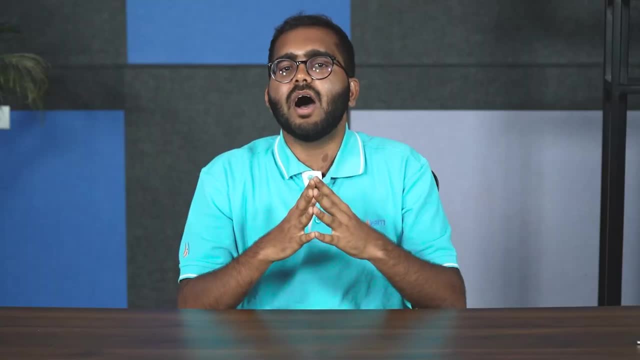 customer satisfaction, boost income and acquire a competitive space in the market. Many studies show that AI will create about 97 million jobs in the upcoming years. Let me tell you how Simply Learn can help you master AI. Make sure to check out the Professional Certificate Program on AI and. 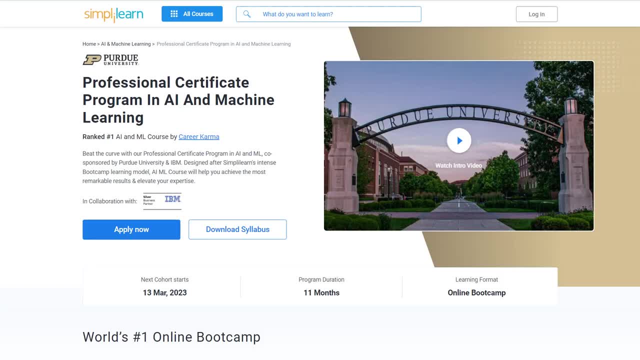 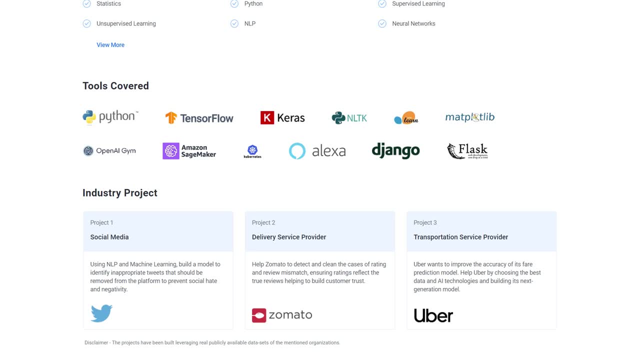 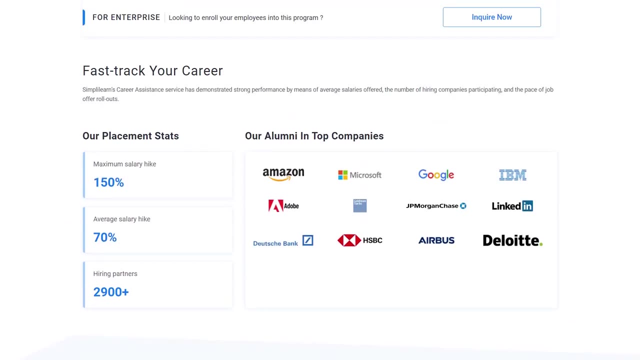 Machine Learning in collaboration with Purdue University and IBM. You can fast track your career by learning tools like Python, TensorFlow, Keras, Django and many more. Our alumni work in top companies like Amazon, Adobe, Google, IBM, Microsoft, Deloitte, and the list goes on and on. 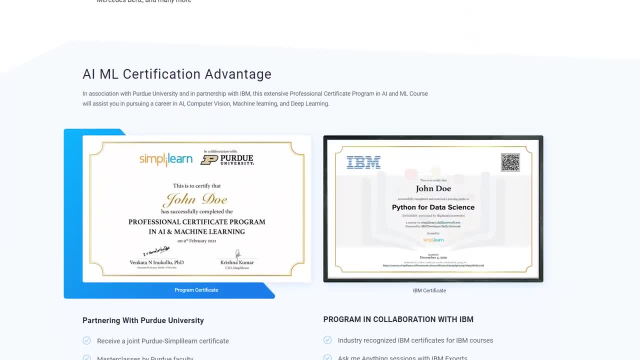 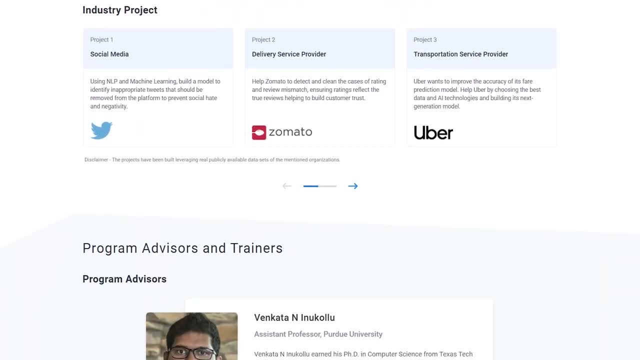 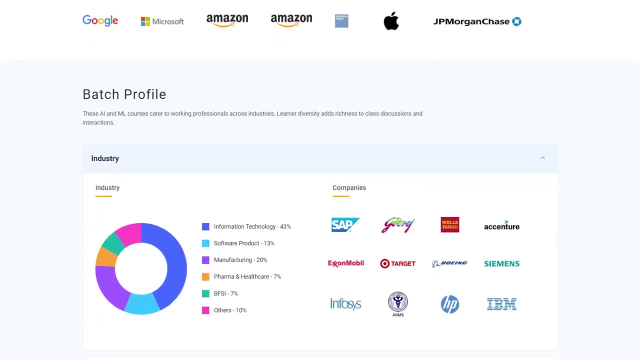 Start an exciting, lucrative career in the field of artificial intelligence with our Professional Certificate Program in AI and Machine Learning, in collaboration with Purdue University and IBM. for growth, innovation and fulfillment. Enroll now to start your journey towards a rewarding career today. Link is in the description and pinned comment After watching this full course.